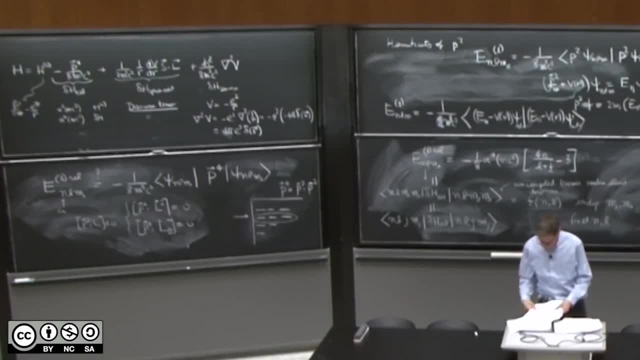 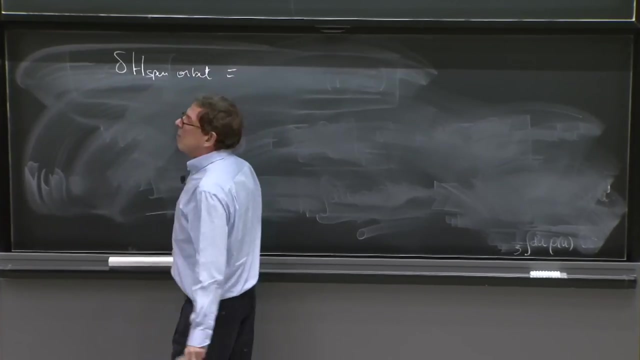 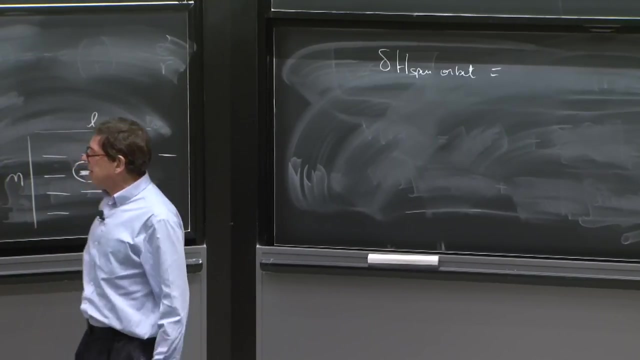 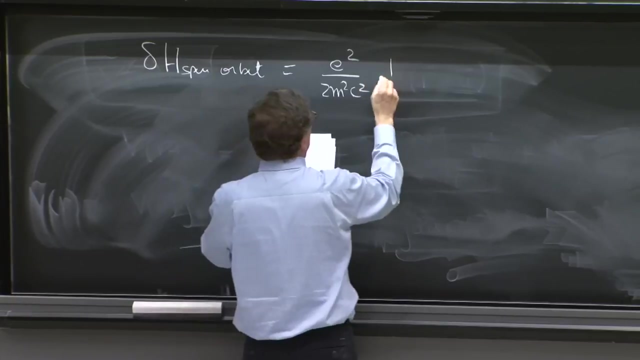 All right, Spin orbit. We have it still there. delta h spin orbit. Well, we know what v is, so that derivative dv dr can be taken care of. the 1 over r, That gives you e squared over 2, m squared, c squared 1. 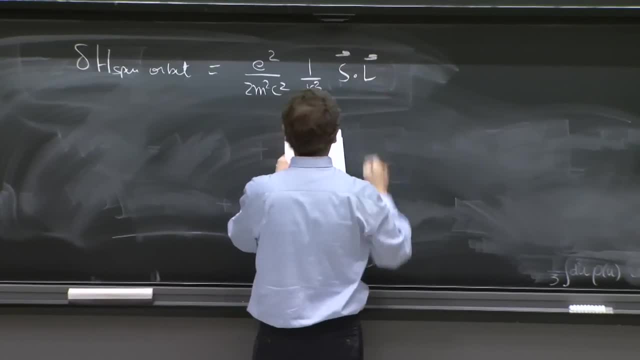 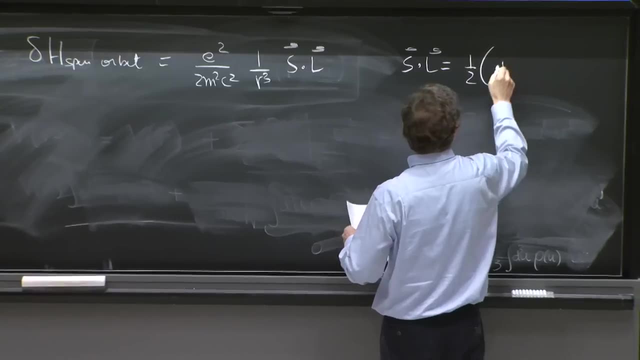 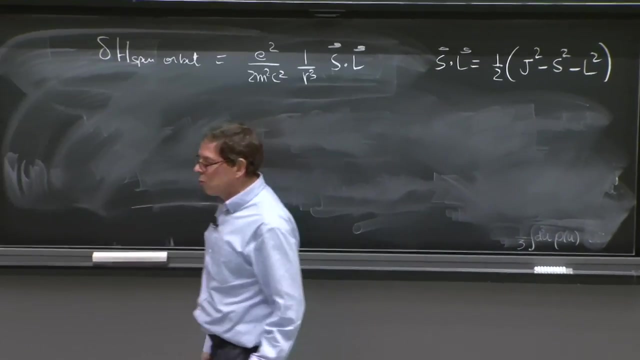 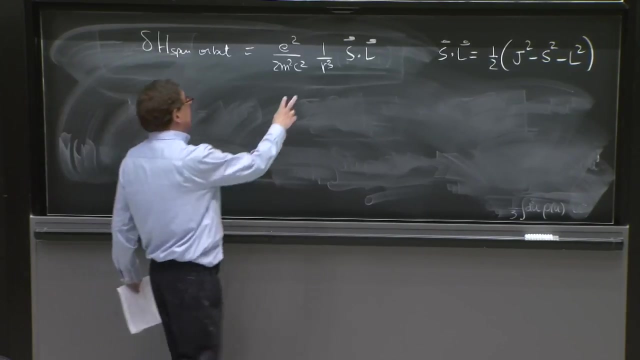 over r cubed sl And you remember that sl from 805, j squared minus s squared minus l squared. The reason that's why you tend to do addition of angular momentum, Because The s and l calculating the matrix elements of this thing. 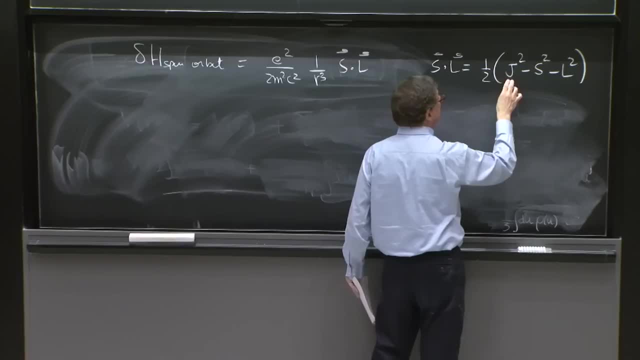 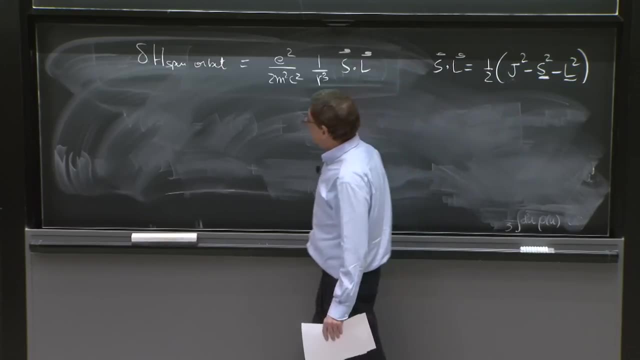 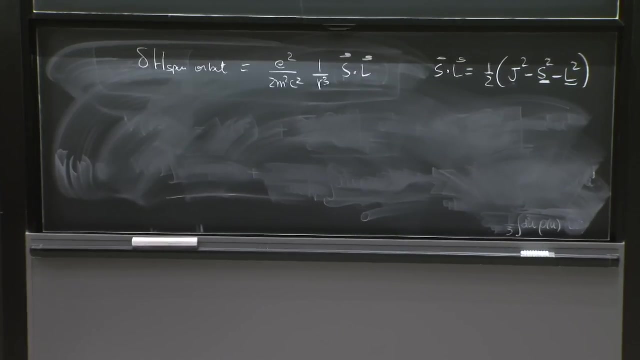 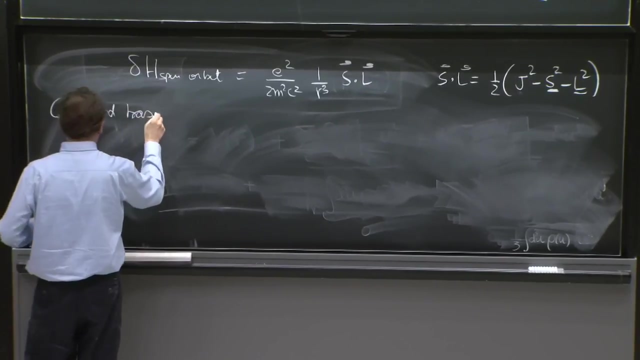 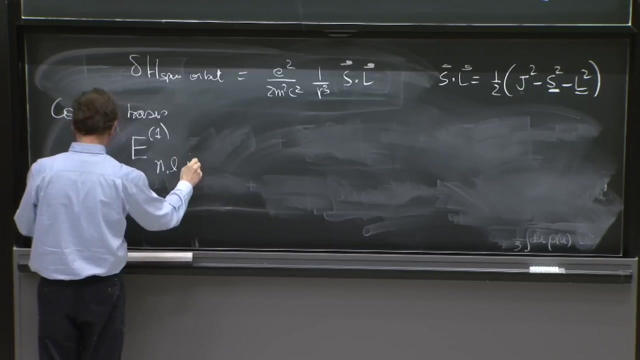 is very easy in that basis, Because every state there has a fixed value of s squared, a fixed value of l squared and j squared has a couple of possibilities. So we must work with the coupled basis And therefore we can attempt to find e1 of n, l, j, m, j. 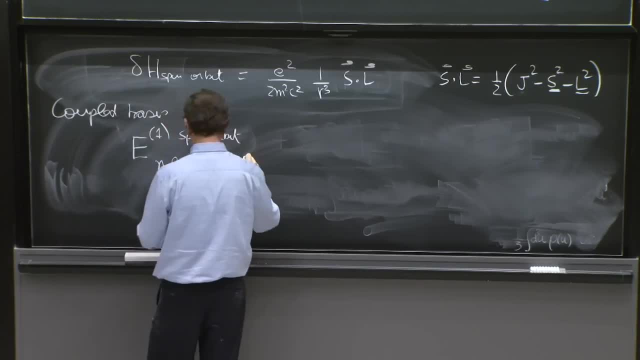 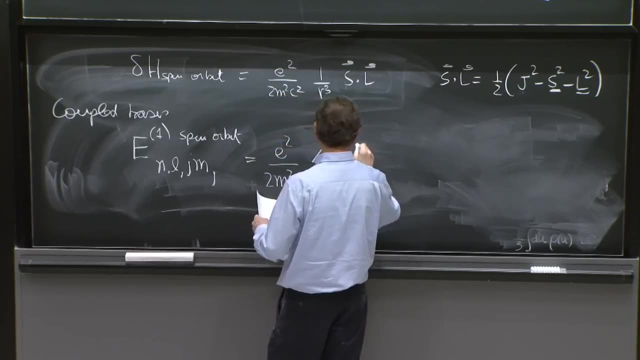 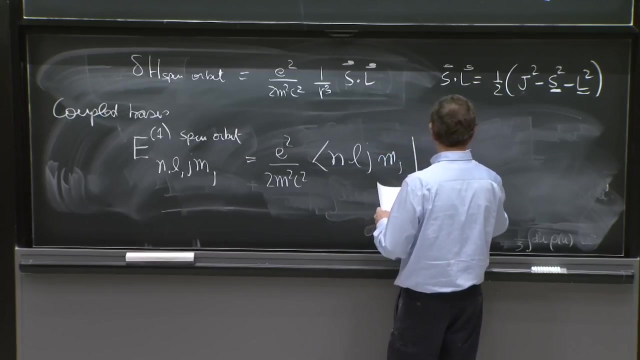 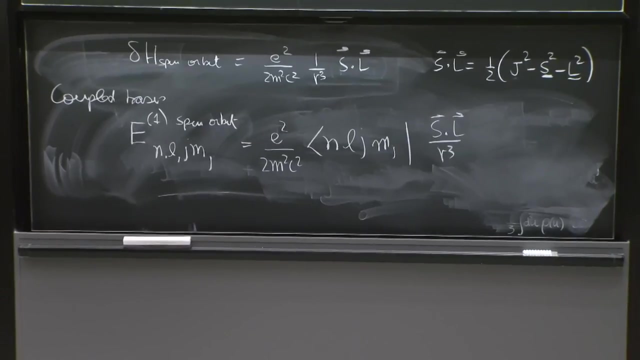 spin orbit equal e, squared over 2 m, squared c, squared n, l, j, m, j, s, l, r cubed. The r cubed has to stay inside, Right Inside, the expectation value, because the expectation value includes integration over space. 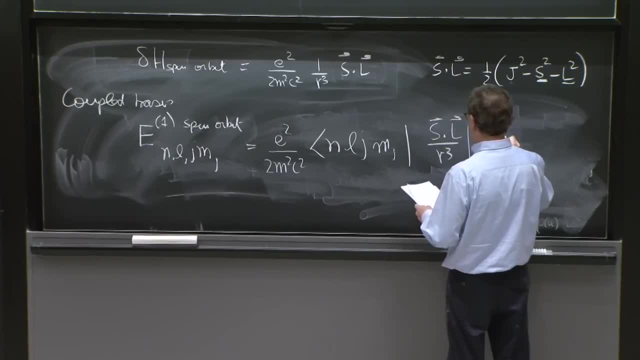 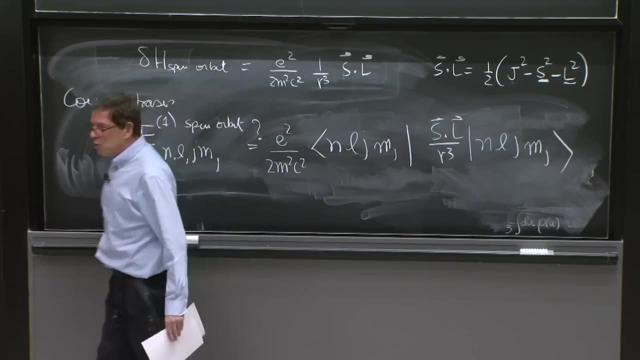 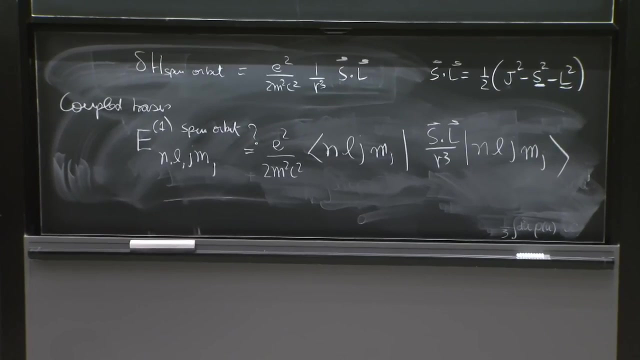 So this is very important: n, l, j, m, j And again the usual question: The coupled basis will have degeneracies. All the states are degenerate there. So this time we fixed n, because degeneracies happen only. 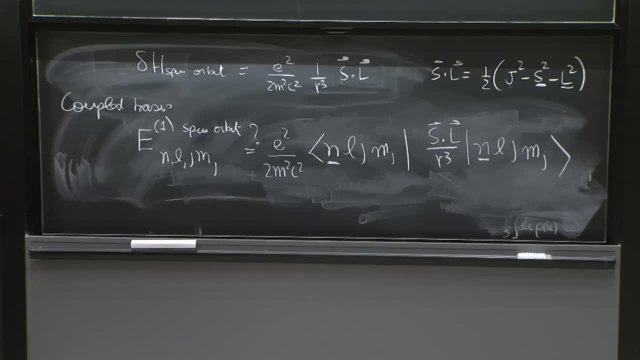 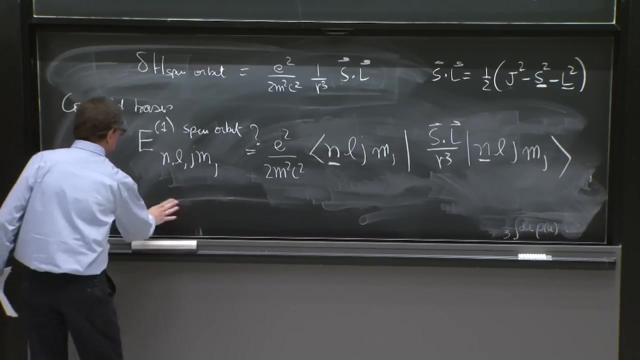 when you fix n, So do we have the right to do this, to use the formula for perturbation, the non-degenerate perturbation theory, to do this calculation? And the answer is yes, because the perturbation s dot l over r. 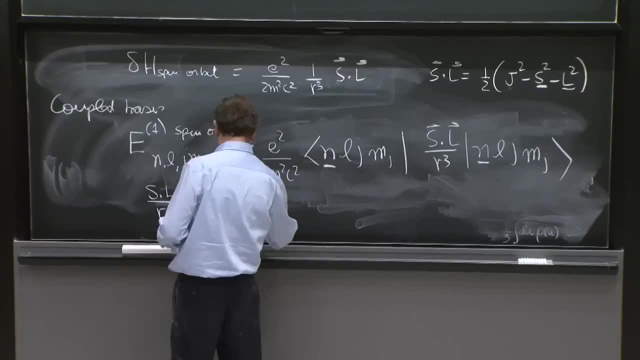 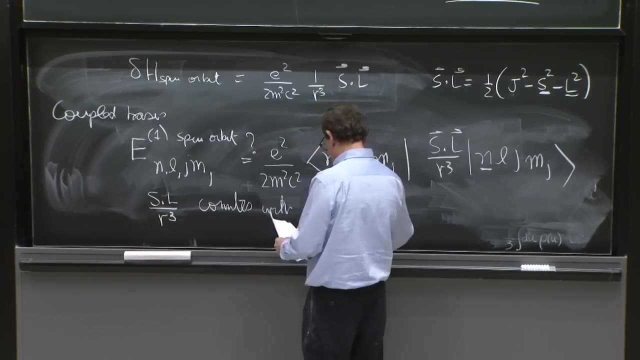 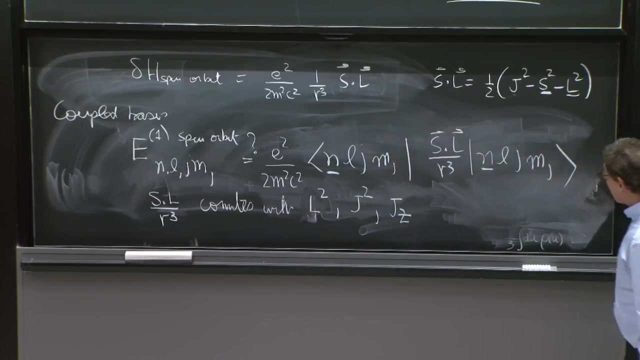 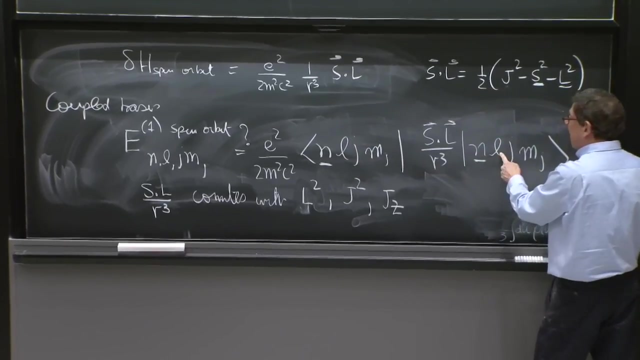 cubed, So we can commute with l squared, with j squared and with jz. OK, you need all that because you can have degeneracies by having different l values And that would be taken care by this operator that has different. 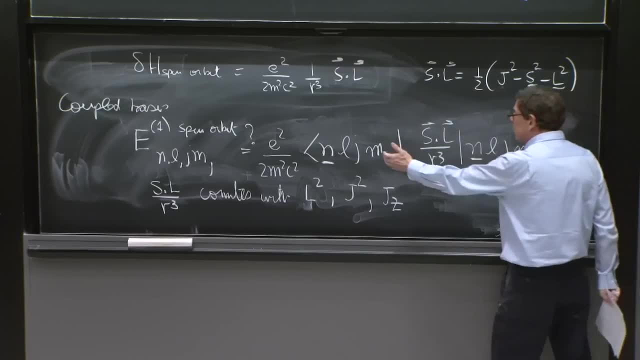 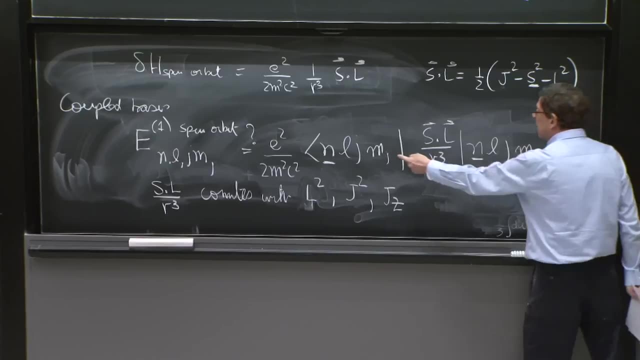 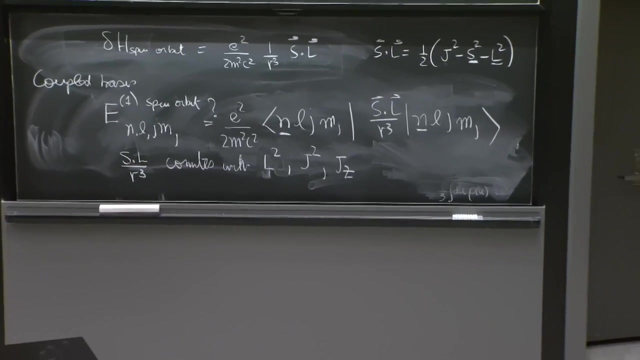 values. You can have degeneracies involving different j values. This would be taken care by this operator. And you can have degeneracies when m has different values, So that involves the jz operator. So you really need a perturbation that commutes with all of them. 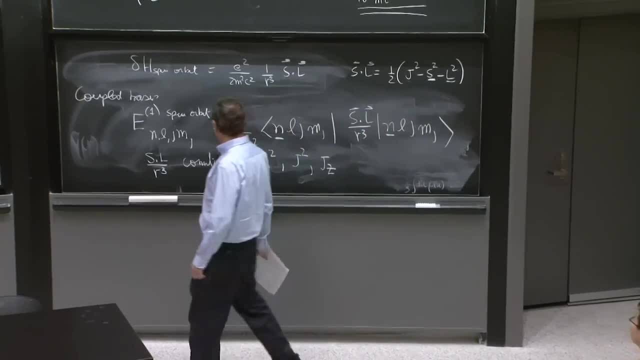 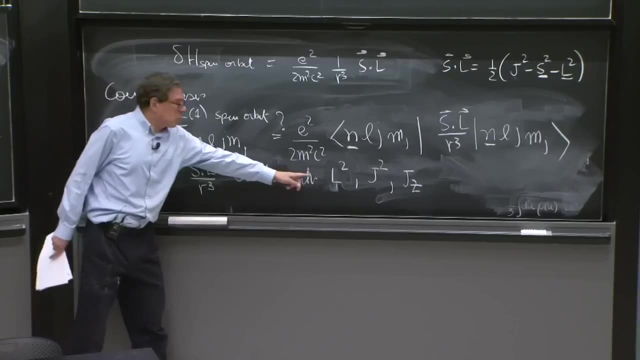 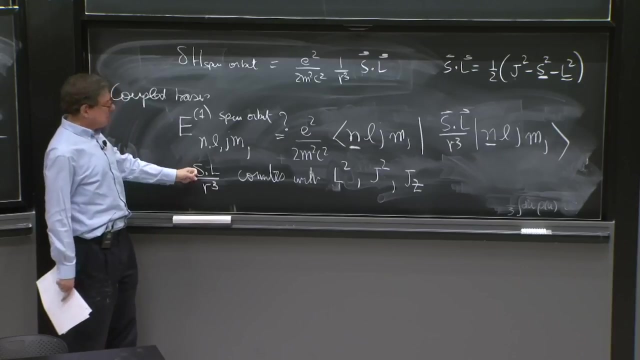 And why does it commute with all of them? So you can see it in several ways. Let's do l squared. l squared is Casimir. It commutes with any li. It doesn't even think about s because it doesn't know. 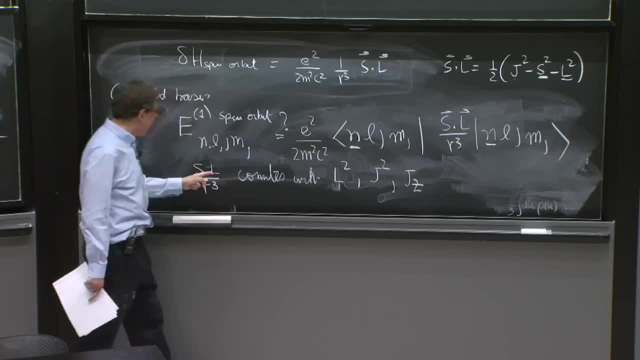 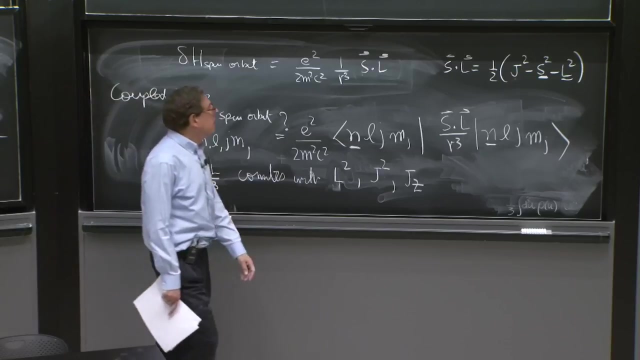 anything about s, so it commutes with s. So l squared commutes with any li and it commutes with s And l squared is an invariant commutes with r squared because r squared is rotational invariant, So everything commutes with that. 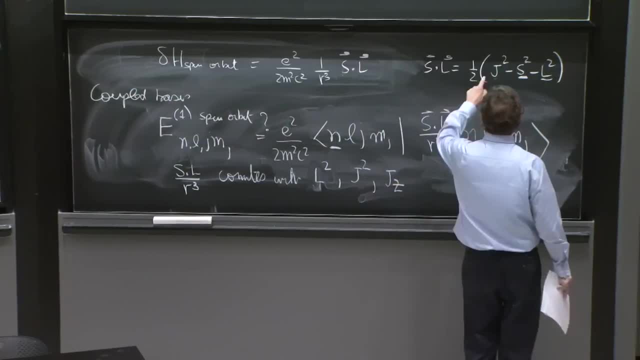 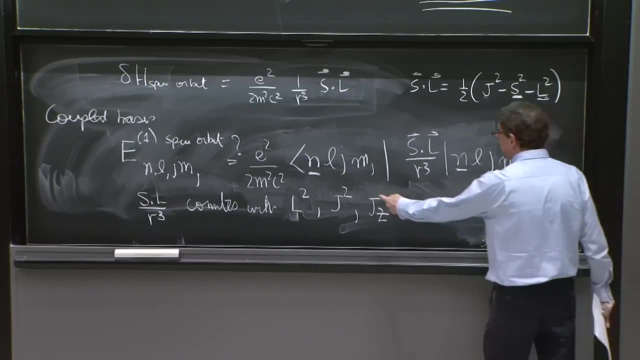 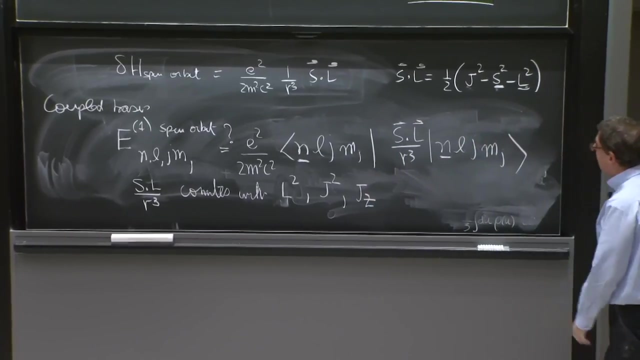 In order to do the other ones. you can also think in terms of this matrix, j squared over here and s squared and do all of them. You should do it and convince yourself that they all commute. So we can do this. 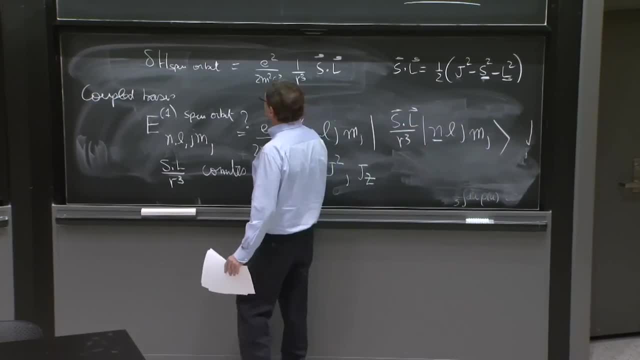 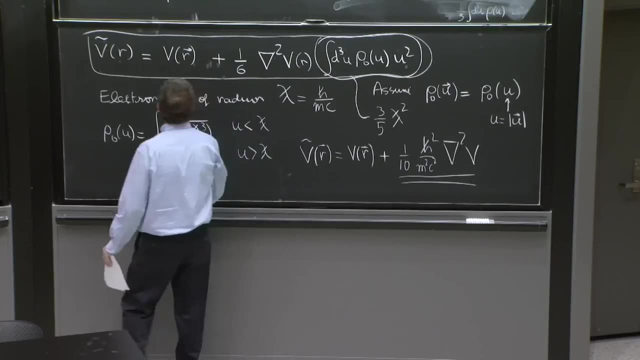 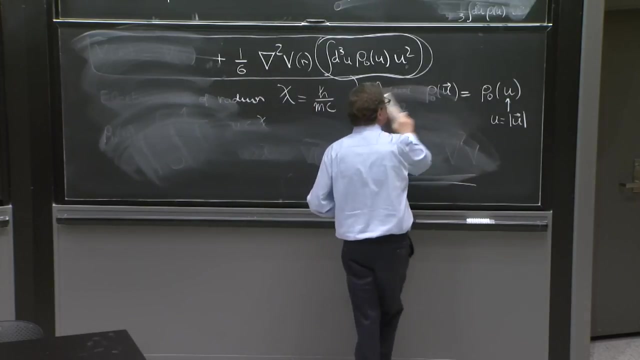 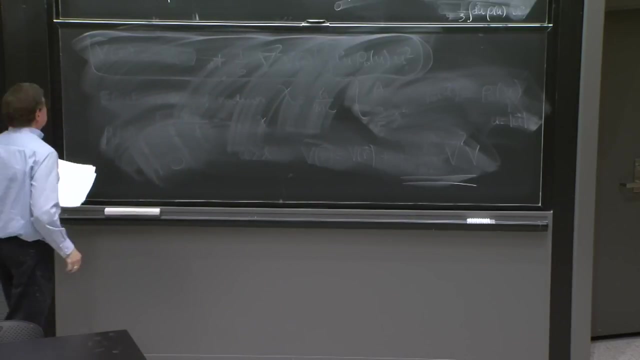 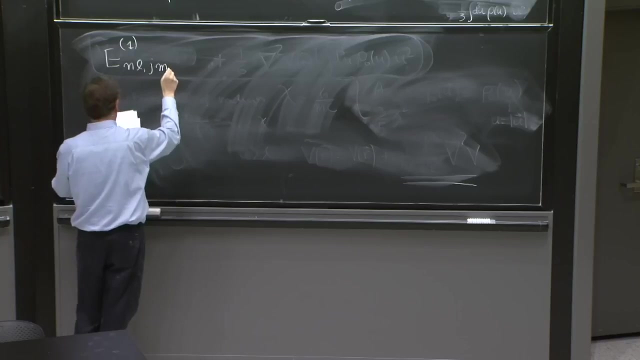 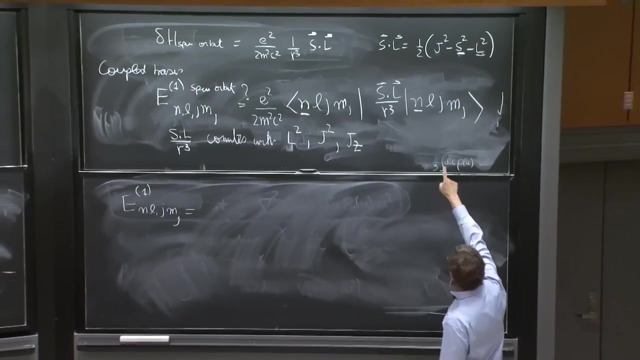 And if we can do it it's good, because then we can evaluate these quantities. So let's do a little of the evaluation. So this e1nlj1. Let's say mj is equal to. let's evaluate the sl part. 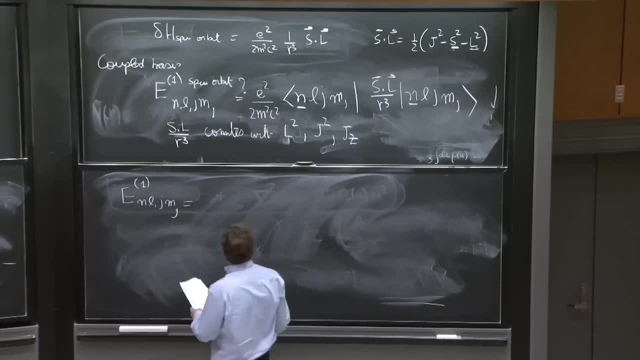 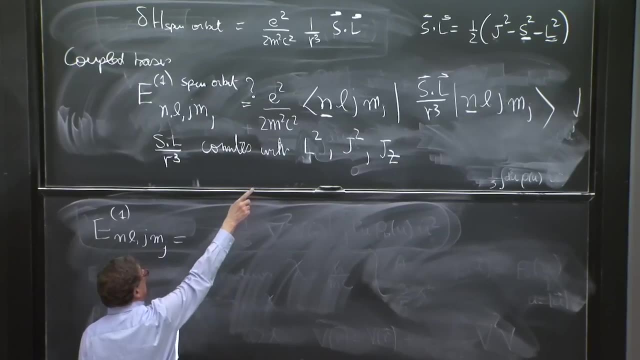 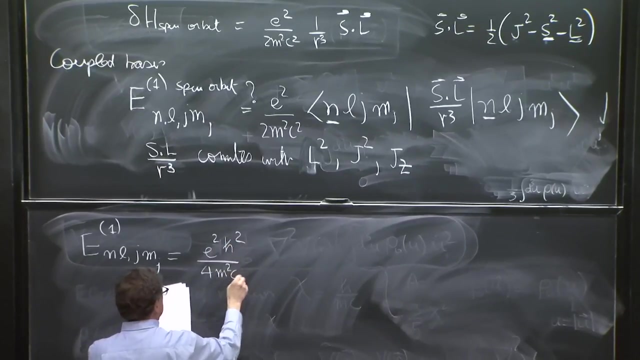 by using 1 half j squared, s squared minus l squared, So that gives you a factor of h bar squared over 2, with this 2 over there, So you get e squared, h squared over 4, m squared, c squared, j times j plus 2.. 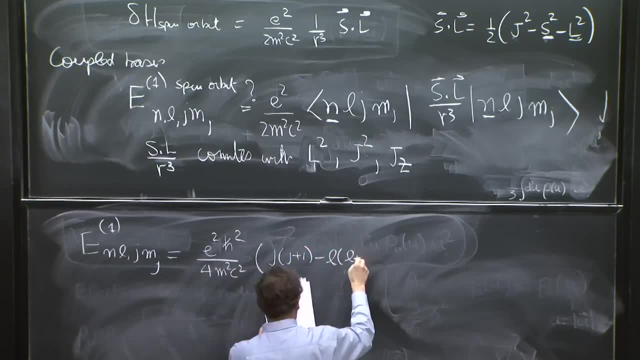 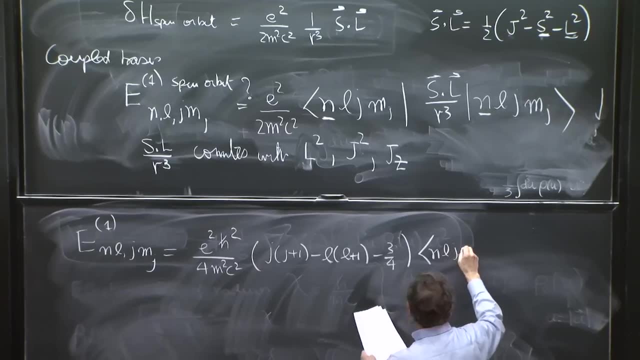 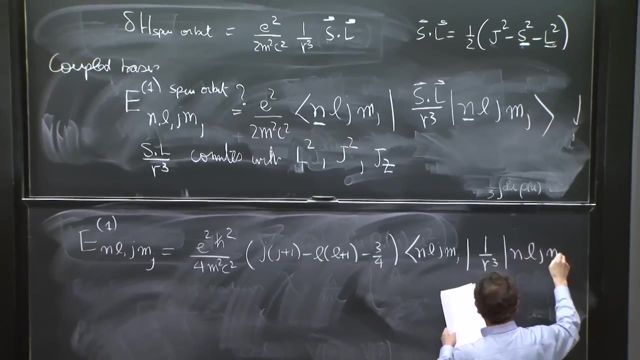 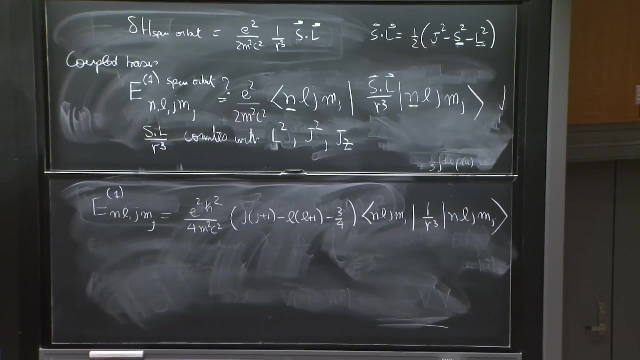 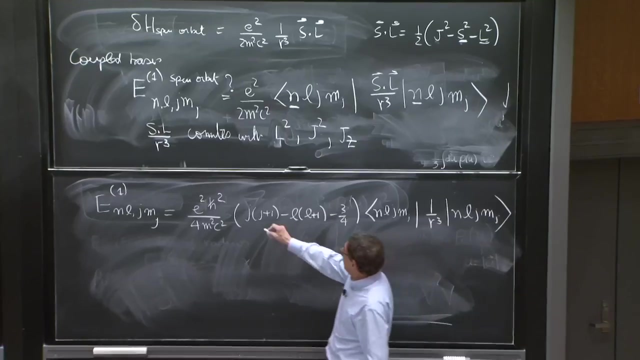 So you get e squared, h squared over 4 m squared, c squared. So you get a plus 1 minus l times l plus 1 minus 3 quarters times nlj mj. 1 over r cubed nlj mj. OK, That should be clear from the fact. 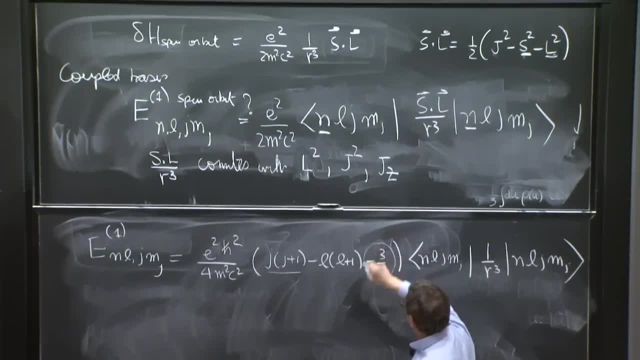 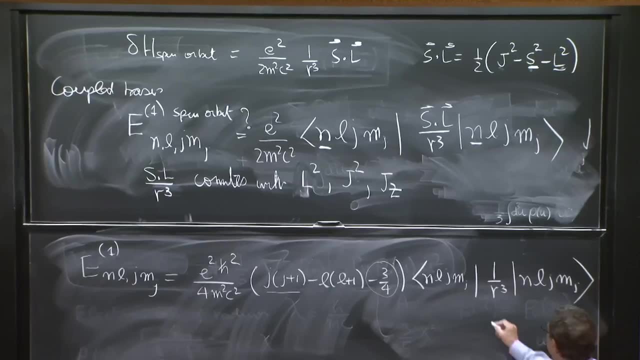 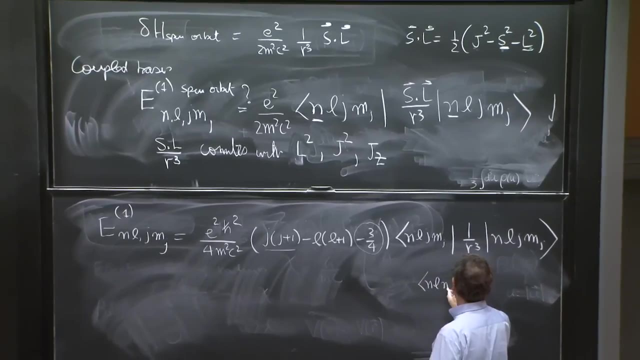 we have a j squared minus s squared, That's a 3 quarters. Spin is always 1 half And l squared. This is known. It's equal, in fact, to nlml 1 over r cubed nlj OK. 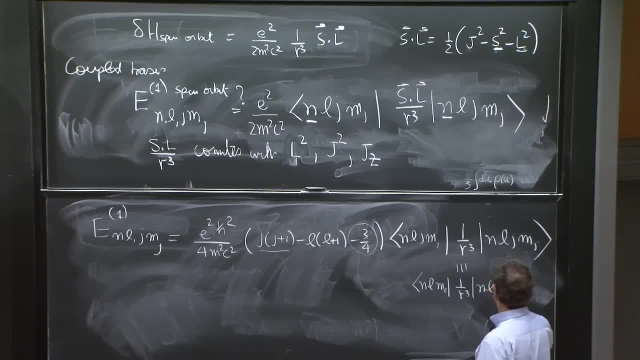 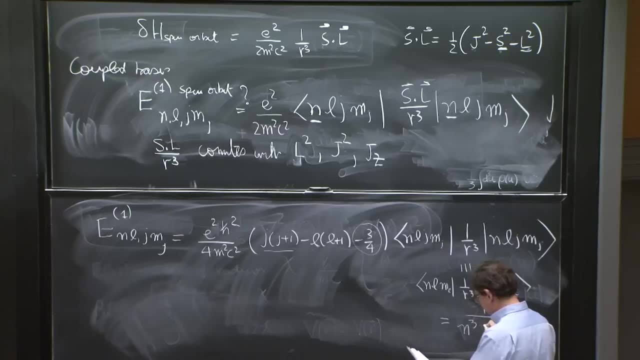 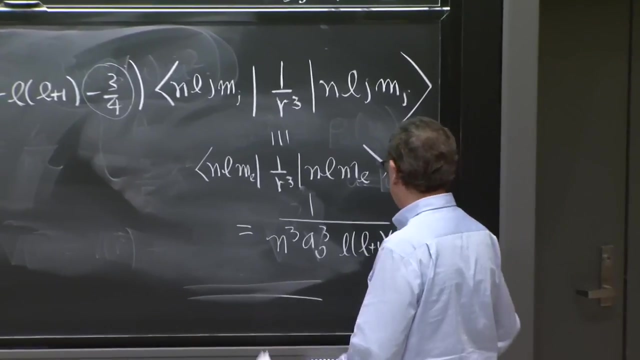 That's a 3 quarters. Spin is always 1 half And l squared, And l squared is equal to ml, which is equal. let me discuss that again. It's a little a0, l, l plus 1, l plus 1 half. 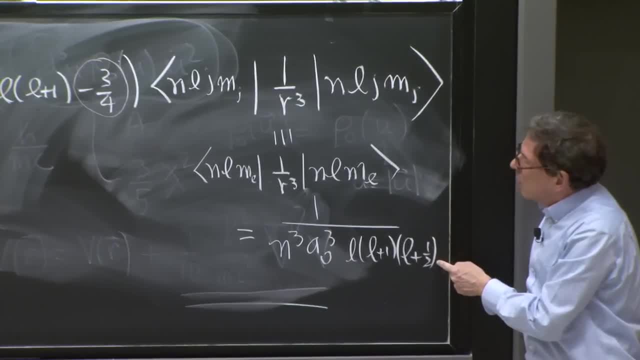 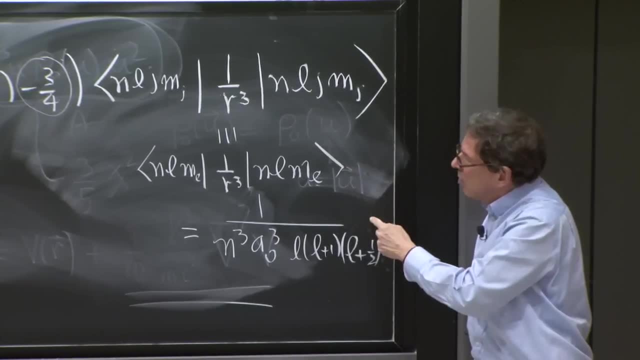 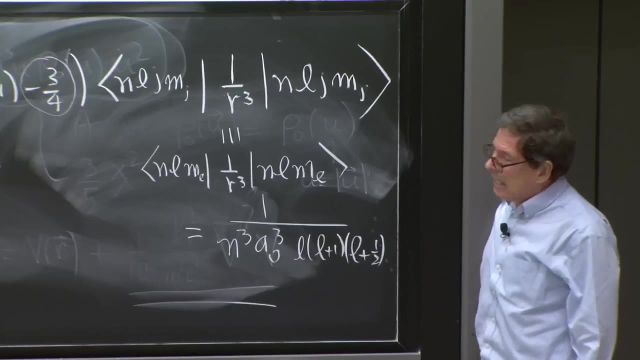 OK, So this is a known result. It's one of those expectation values that you can get from Feynman-Hellman or for other recursion relations. was computed in the original uncoupled basis. We seem to need it in the coupled basis.